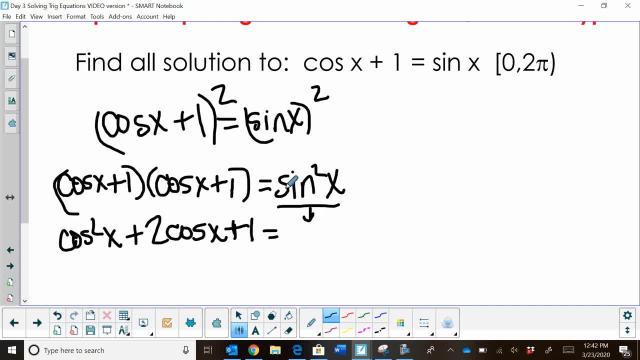 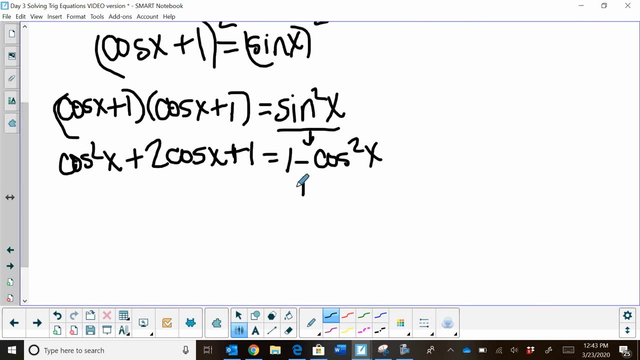 we want to convert this to one trig function, So I'm going to use the Pythagorean identity: 1 minus cosine squared x. Now I've got everything in terms of sines and cosines. Everything's in terms of cosine. Now let's combine our like terms. 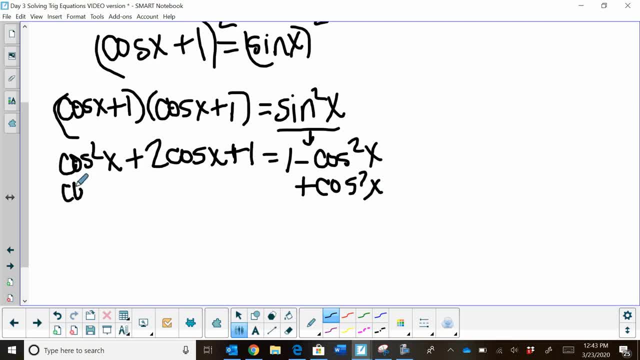 And I'm going to add cosine squared x to both sides And I'm going to subtract 1 from both sides. So what are we left with? We're left with 2 cosine squared x plus 2 cosine x, And then this zeroes out, so equals 0.. Now this left side. I can factor. 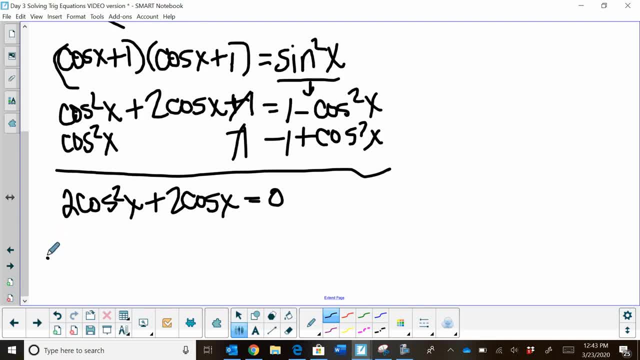 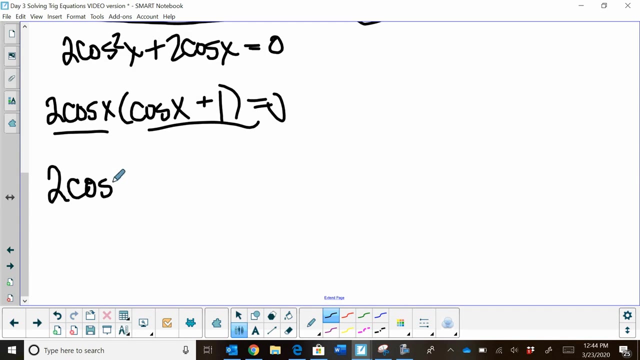 I have a GCF of 2 cosine x. So I'm going to factor out my 2 cosine x And I'm left with cosine x plus 1 equals 0. And then set each one equal to 0. Once you factor, you've got when is cosine of x equal to 0? And when is cosine x plus 1 equal to 0?. 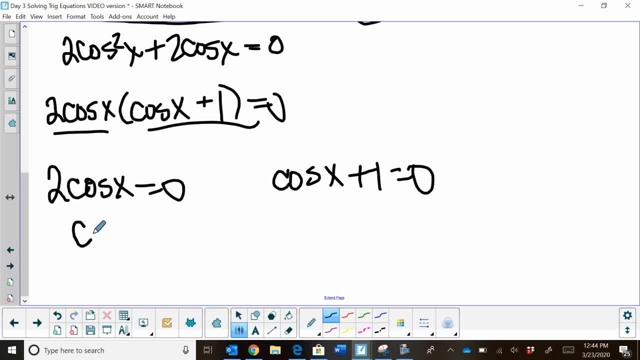 So this left side just divide both sides by 2. So you just get cosine x equals 0.. What angle is cosine 0?? We know that's at pi halves and 3 pi halves on the interval 0 to 2 pi. 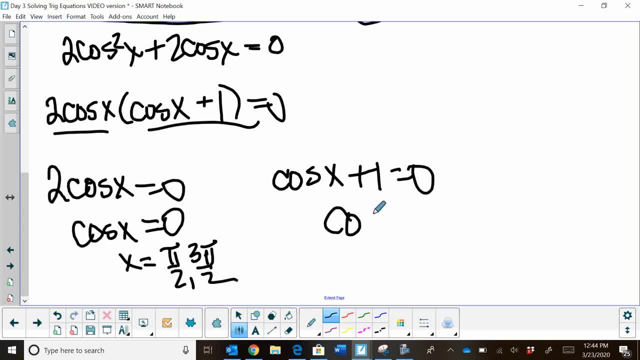 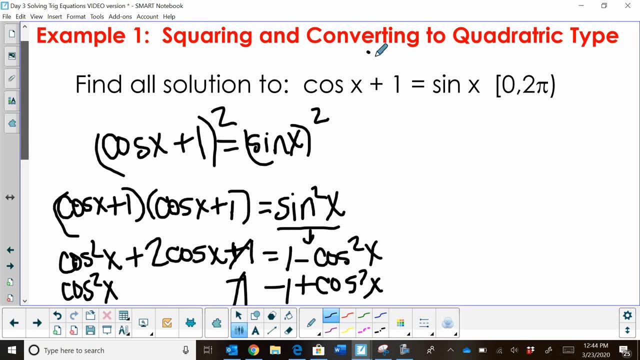 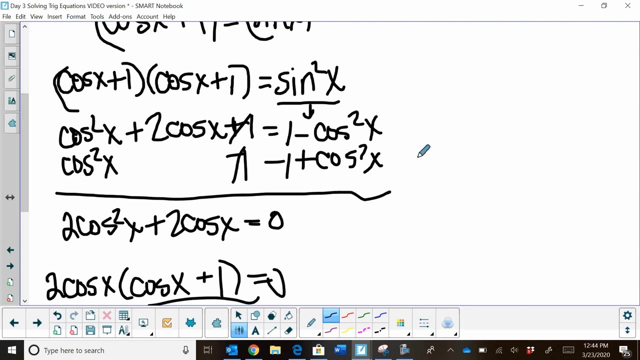 And then when is cosine negative 1, cosine x negative 1, we know that's when x is pi. So there we go. We have those three solutions For this equation on the interval 0 to 2 pi. So what do we do? We squared both sides and then we were able to convert it to just a factoring quadratic. 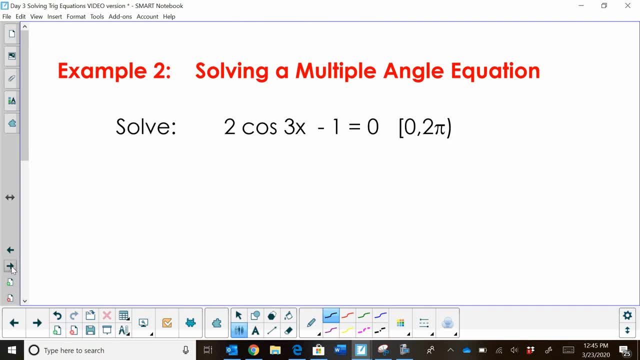 OK, so let's look at a second one. This one involves multiple angles. OK, how do you recognize multiple angles? Well, there's a coefficient in front of your angle. So in this case we've got cosine of 3x. 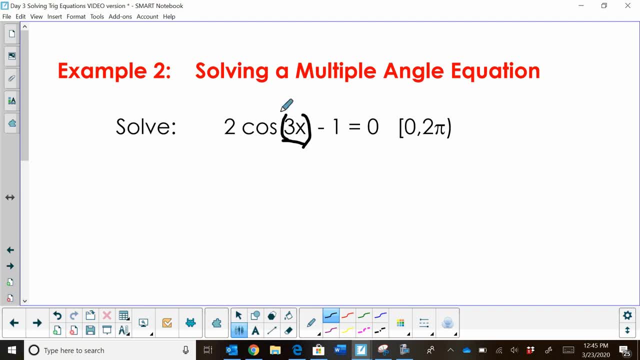 So how you're going to solve it is you're just going to kind of ignore the fact that you have a multiple angle in the beginning and just solve it like you. we've been solving these. So we're going to take cosine or 2: cosine of 3x minus 1 equals 0.. 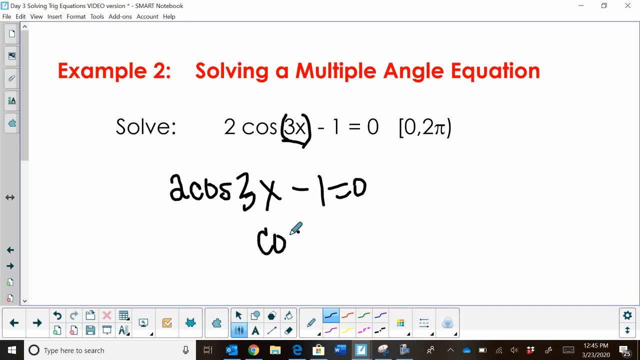 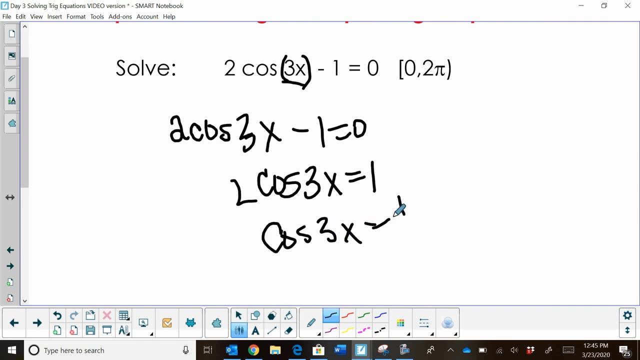 We're going to add 1 to both sides, So cosine- I'm sorry- 2 cosine of 3x is equal to 1.. Divide both sides by 2 cosine, So cosine of 3x is equal to 1 half. 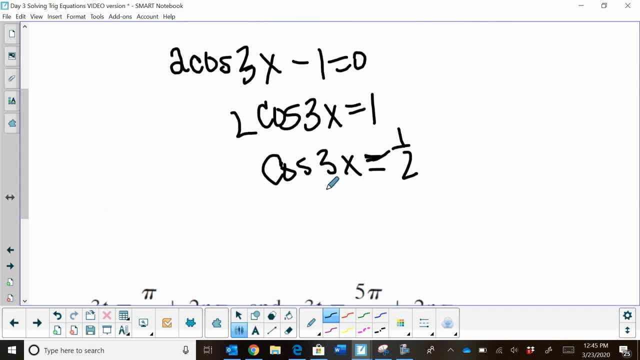 OK, now this is where it changes slightly. OK, we're going to identify what positions cosine is equal to 1 half. Sorry, making a little more room here. Well, cosine is 1 half, Let's think about that. It's right here at pi. thirds: 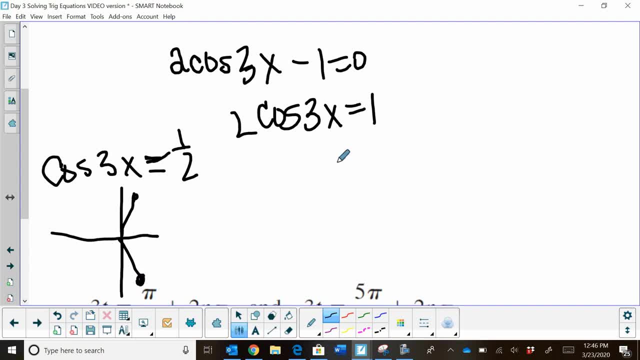 And right here, It's right here- at 5 pi thirds. So we're going to set the angle of 3x equal to a pi thirds. We're also going to set the angle 3x equal to 5 pi thirds, Because those are the answers. 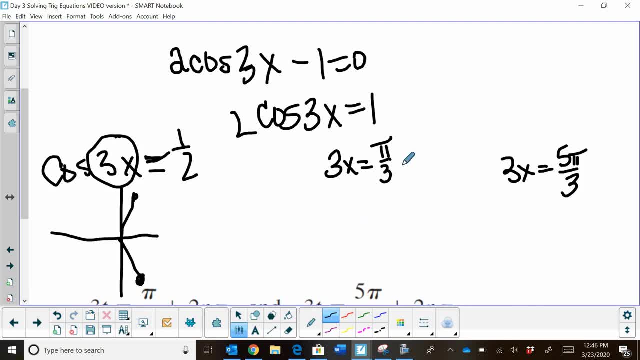 Now what you've got to do here is you have to consider The period of cosine. The period of cosine is 2 pi n OK, which is all the recurring solutions. You're going to set your angle 3x, equal to not only that angle but recurring angles. 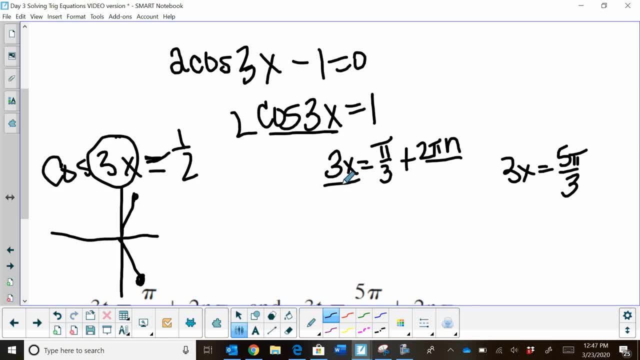 Then we're going to divide both sides by 3, which is the same as multiplying by 1 third, right? So multiply everything by 1 third And what we're going to end up with is: x is equal to. this part becomes pi ninths plus 2 thirds pi n. 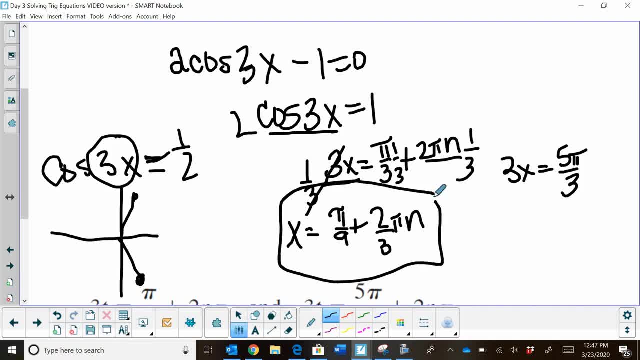 And there's one of our general solutions. The next one. I'm going to do the same thing. I've got 3x is equal to 5 pi thirds. I'm going to add the cycle of 2 pi n to that for my general solutions. 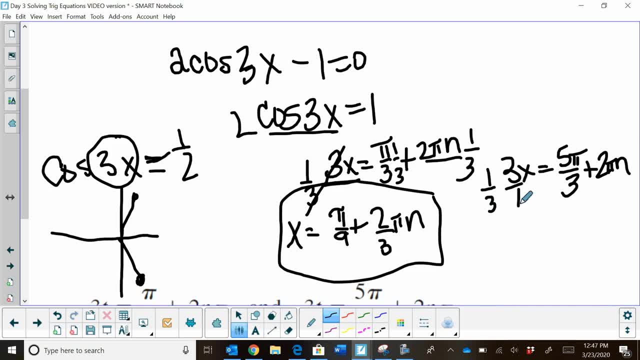 I'm going to then multiply by 1 third, which is the same as dividing by 3.. So multiply each part by 1 third And that gives me x is equal to 5 pi ninths plus 2 pi n, All over 3.. 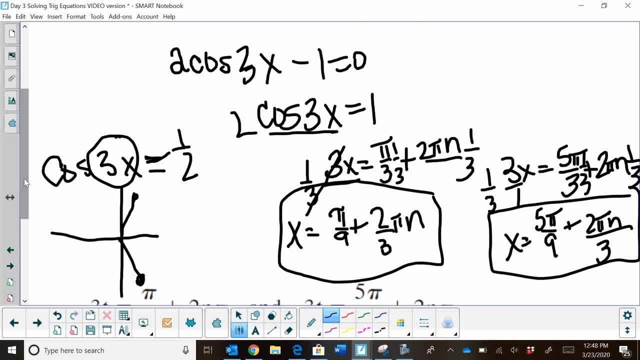 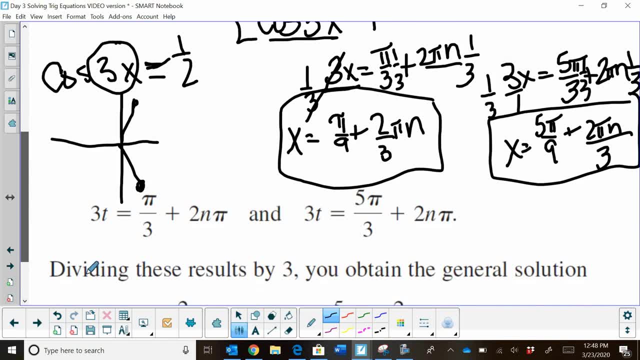 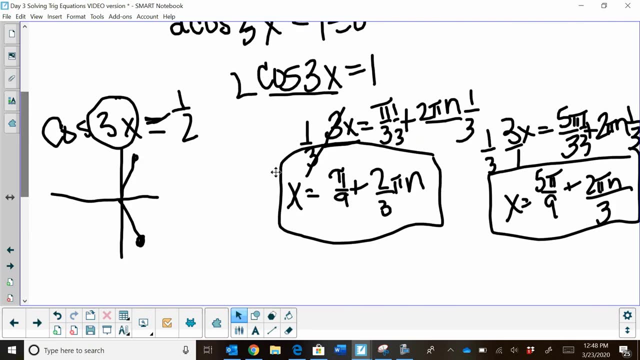 And those are our solutions. Now, if we want to know the solutions on the interval 0 to 2 pi, we then take our general solution and we just list them all. So if you're asked for general solutions, you're done. 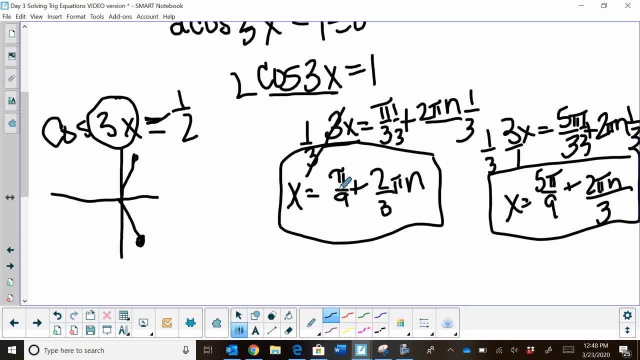 If you're asked for solutions on the interval 0 to 2 pi, what we're going to do is just list them all. So let's list all of them that occur. So the first one, of course, is pi ninths. 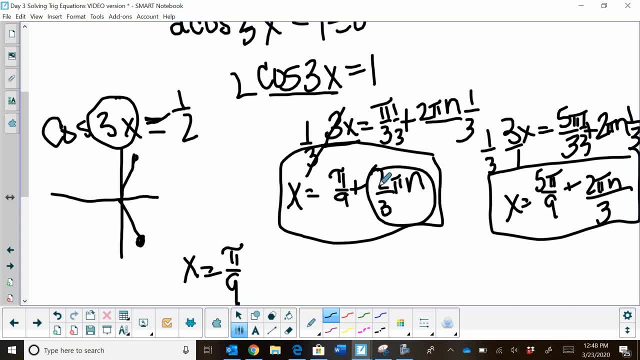 Now I'm going to add a 2 pi thirds to that, which is in the form of: if we multiply top and bottom by 3, that's 6 pi ninths. Okay, So what's pi ninths plus 6 pi ninths? 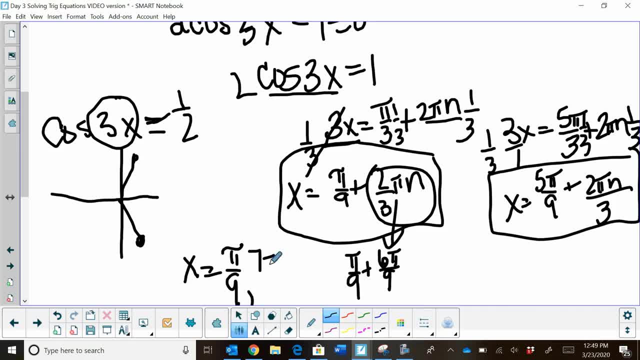 Well, that's 7 pi ninths. That's still less than 2 pi. So let's add another 6 pi ninths, So that would then bring us up to 13 pi ninths. If we added yet another 6 pi ninths, that would bring us to 19 pi ninths. 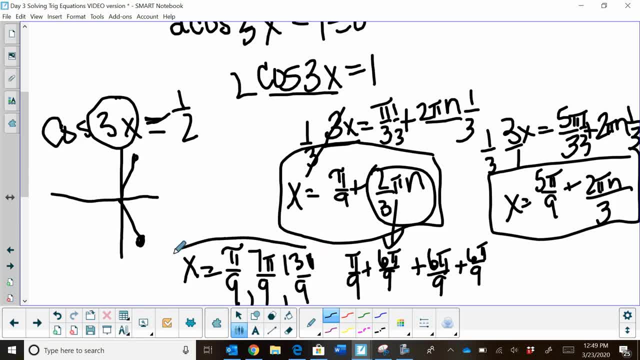 That's outside the unit circle. So it's just these three answers. Now, just to give you a helpful hint: if your coefficient is 3, you're going to have 3 times the number of solutions that you normally would. So pi ninths represented 1, and then we added 2 more, so that was a total of 3 solutions. 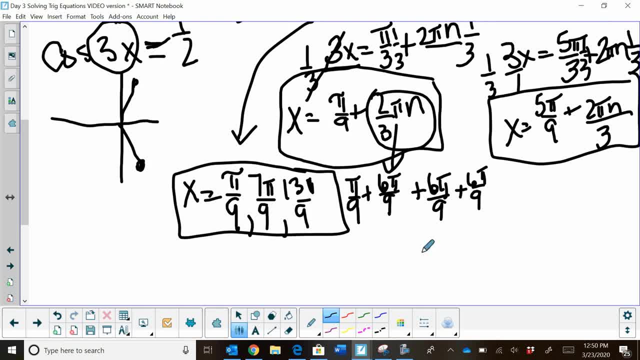 Okay, 5 pi ninths is the first one for this set of answers. Now, because we're dealing with that 3 again, we're going to have 2 more, So let's take. let's take 5 pi ninths and let's add a 6 pi ninths. 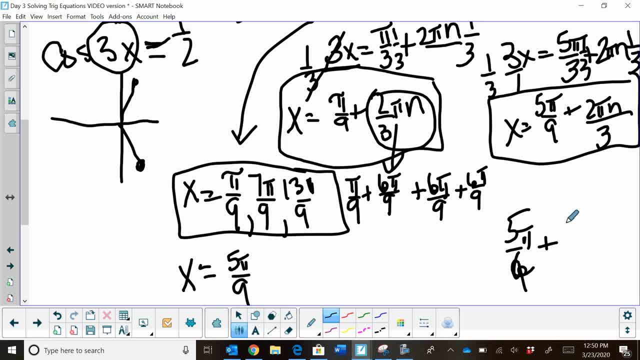 Whoops, I was thinking 6 and wrote: I was thinking 6 and I wrote 6 instead of 9.. So 6 pi ninths And that one's going to give me 11 pi ninths. That is indeed less than 2 pi, because we know 18 pi ninths is 2 pi. 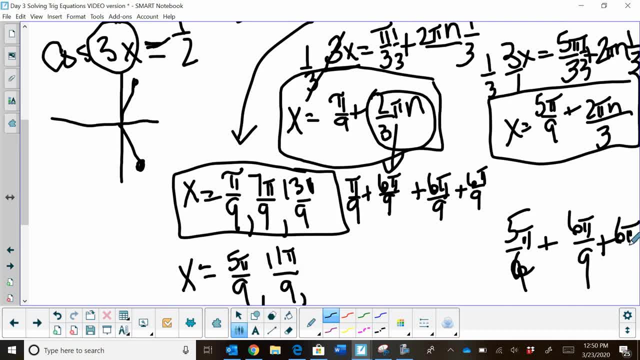 And let's add another 6 pi ninths And that's going to give us 17 pi ninths. That's the last one that falls within the interval 0 to 2 pi. So there we go. This one had 6 solutions. 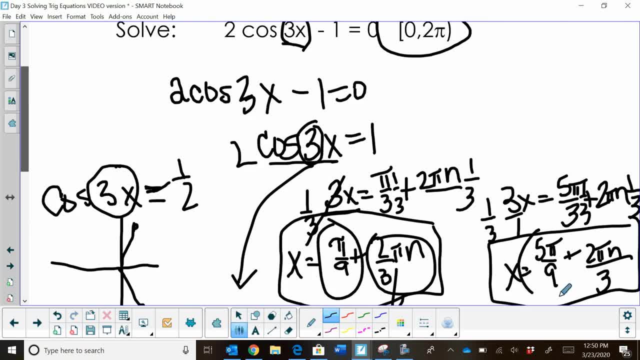 So how could you tell? Well, normally it would have had 2, the pi ninths and the 5 pi ninths. Then we're adding the interval of 2 pi n to it, or actually 2 pi, 2 thirds pi n. 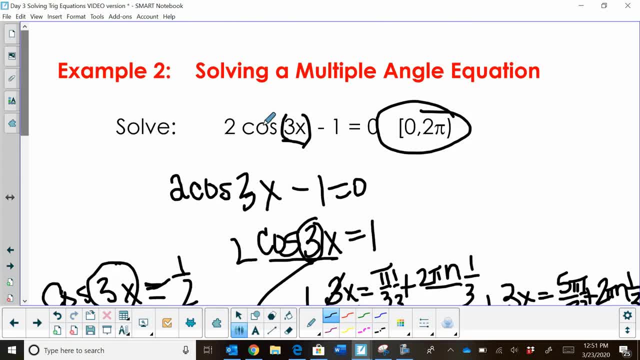 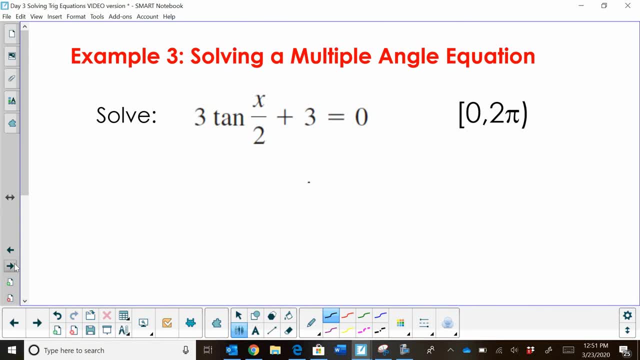 And it created 3 times as many solutions on the unit circle. So that's what this 3 will do. So there you go. So now let's look at a multiple angle, but with tangent. And the reason I wanted to do one with tangent is because we know the period. 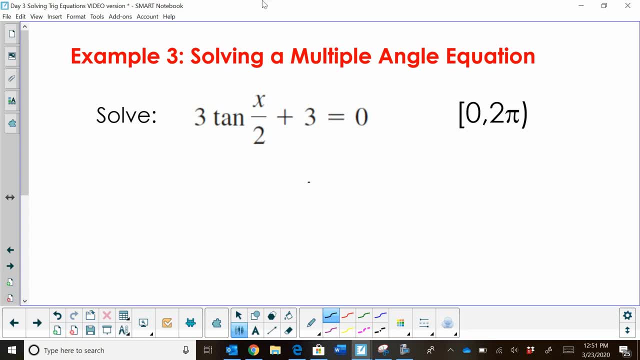 for tangent is pi instead of 2 pi, So it's going to change our answer slightly. So let's go ahead and solve this just like we normally do. So I'm going to subtract 3 from both sides and we're going to get 3 tangent. 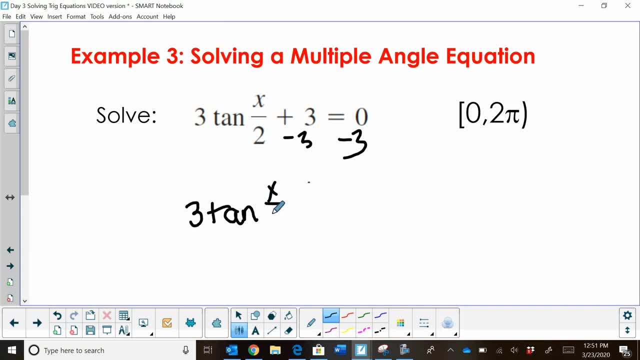 1, pi halves. And notice our multiple angle. this time is not a coefficient, It's not a whole number, It's a fraction, It's half of x. So it's going to change things a little bit. And then tangent of x over 2 is equal to negative 1 by dividing by positive 3.. 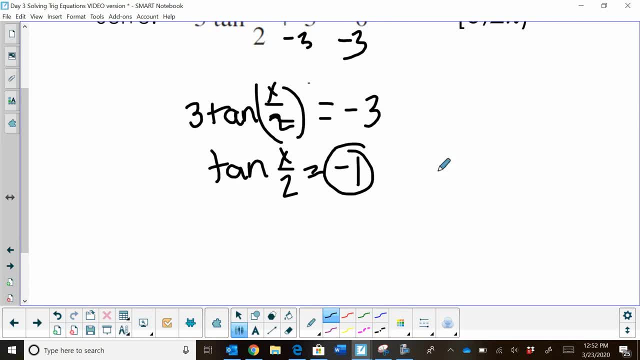 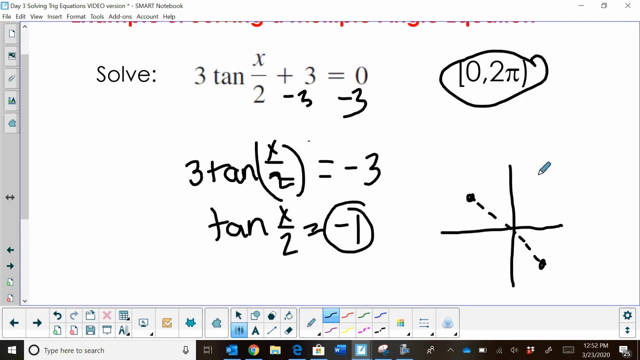 So we need to think about where tangent tangent is negative 1.. Okay, tangent is negative 1 on the interval right here and right here. So, on the interval 0 to 2 pi, we have two positions right. The first one, as we go around the unit circle, is actually at 3 pi. fourths, 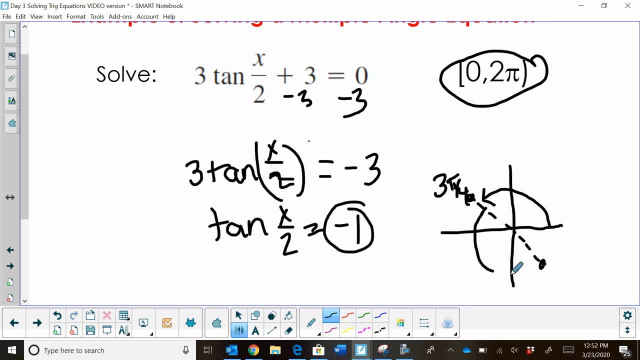 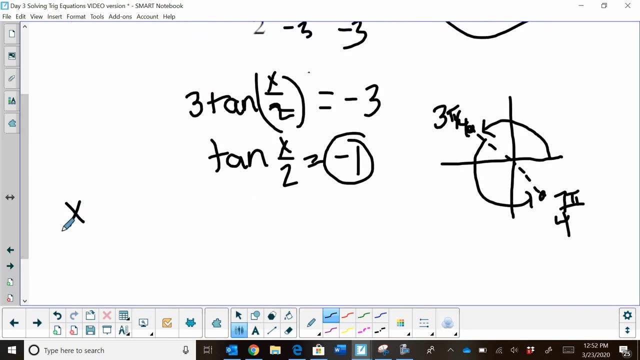 The second one as we go around, the unit circle is at 7. 7 pi. fourths, We want only the answer 0 to 2 pi. So those are the only two we're going to kind of set up. So the first one: let's set up the angle, which is pi halves this time. 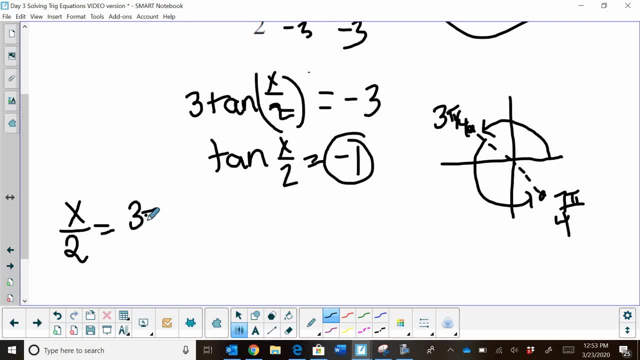 We're going to set it equal to 3 pi fourths And we're going to think about adding pi into it, because then it's going to repeat every pi. right, It's just pi apart. So it actually it counts for this other one over here, because if I take 3 fourths and I add pi into it. 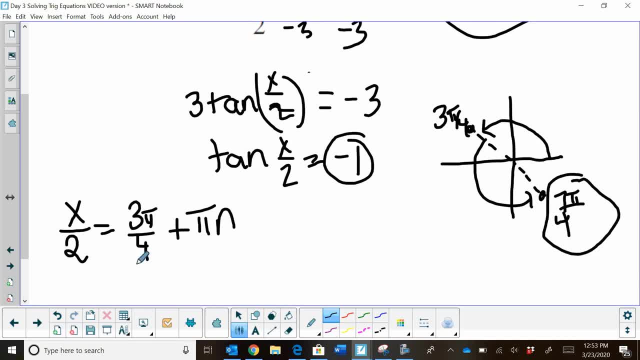 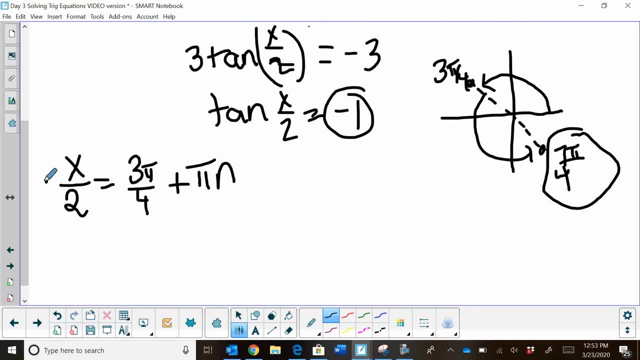 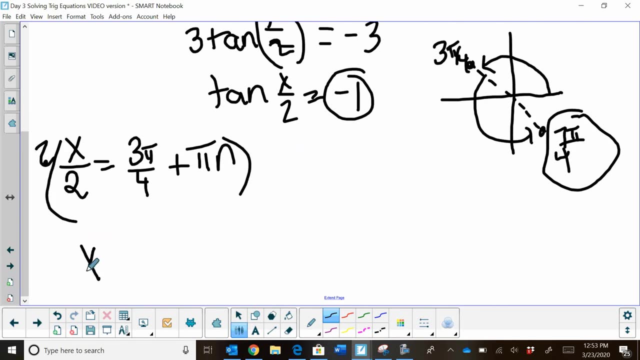 I get 7 pi fourths, So I can just leave that as my answer. Okay, now I need to solve for x. So I'm going to multiply everything by 2 on the both sides, the whole equation by 2.. So x is equal to 2 times 3 pi fourths. 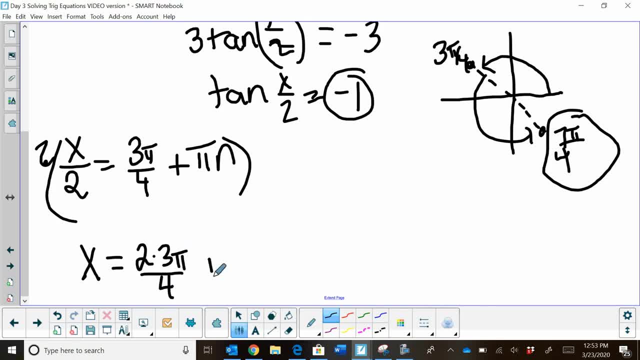 Oops, I didn't get my last line in there- Plus 2 pi n. So that changed this cycle to 2 pi n. Now what's going to happen here is I'm going to end up with 3 pi halves. So my final answer is 3 pi halves plus 2 pi n. 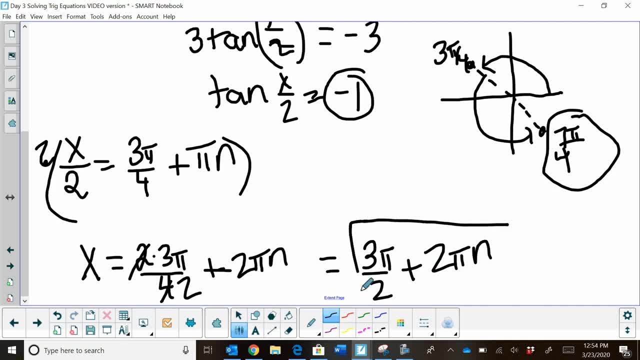 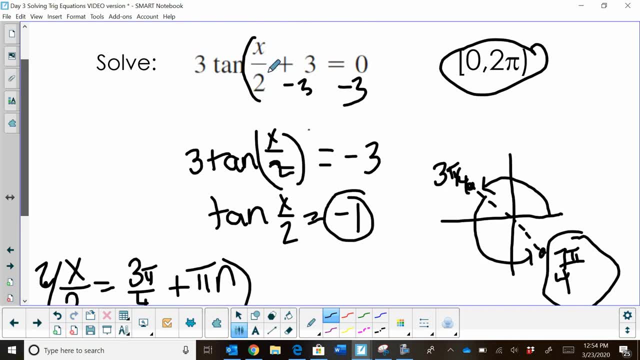 And there's my final answer for x. Now what is happening is, whenever you have a coefficient on your angle- in this case the coefficient was 1 half x- You're going to have half the number of solutions on the interval 0 to 2 pi. 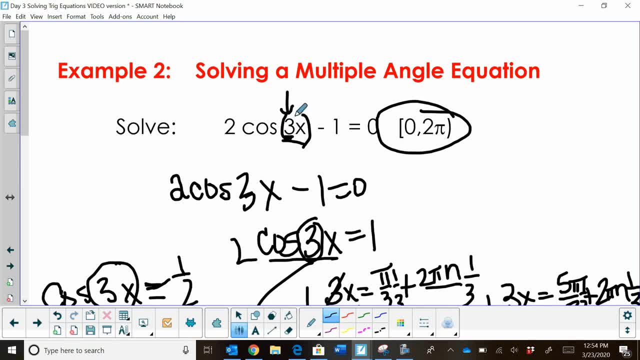 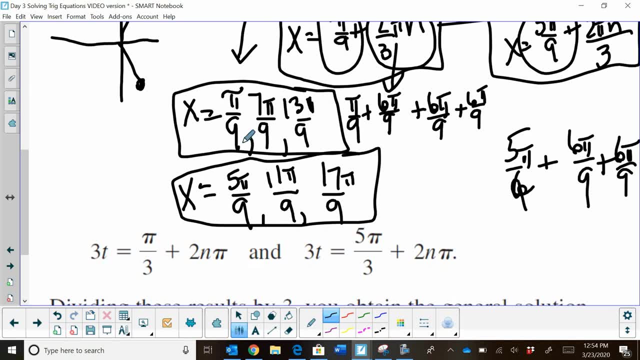 On the other one, we had a coefficient of 3.. You're going to have 3 times the number of solutions on the interval 0 to pi. So this one, it ended up, instead of having 2 solutions, it had 6..